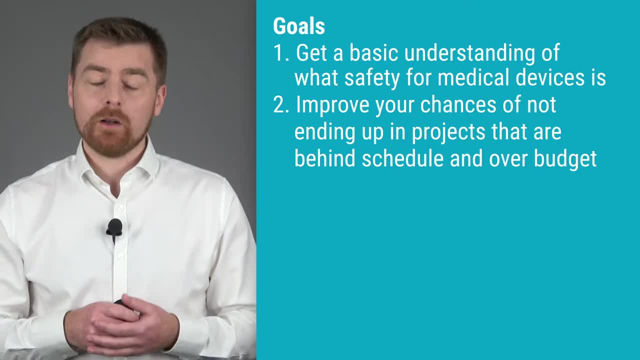 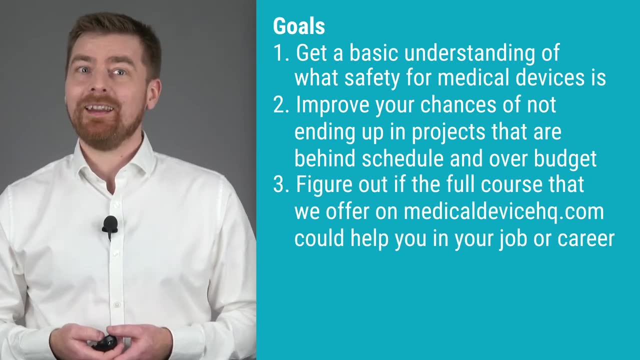 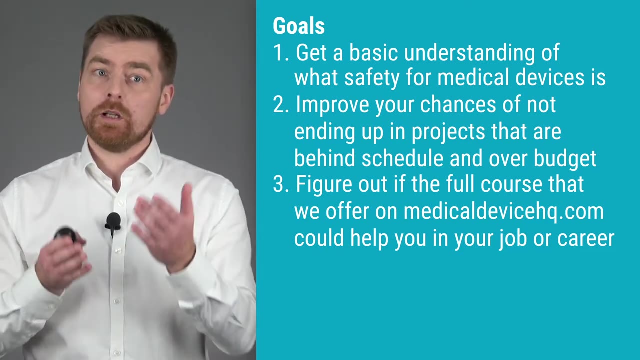 And improve your chances of not ending up in projects that are behind schedule and over budget. Based on that, you should be able to figure out if the full course on safety for medical devices that we offer on medicaldevicehqcom could help you in your job and your career. 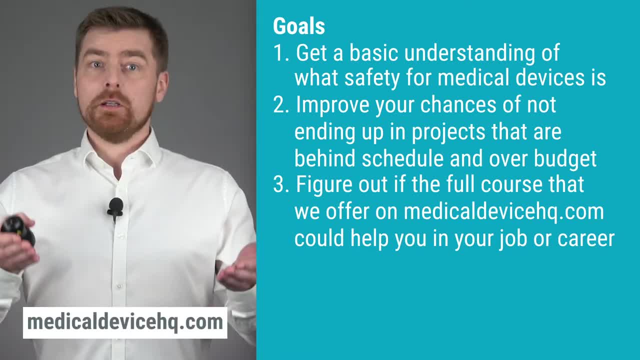 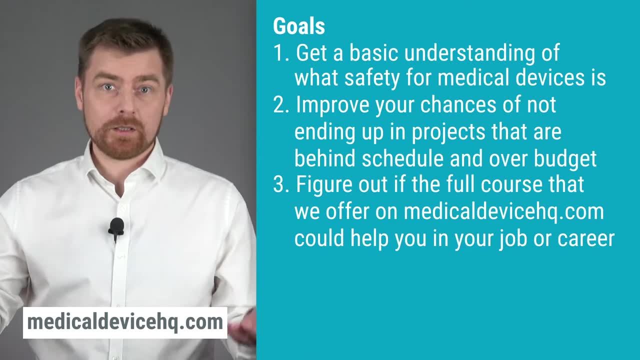 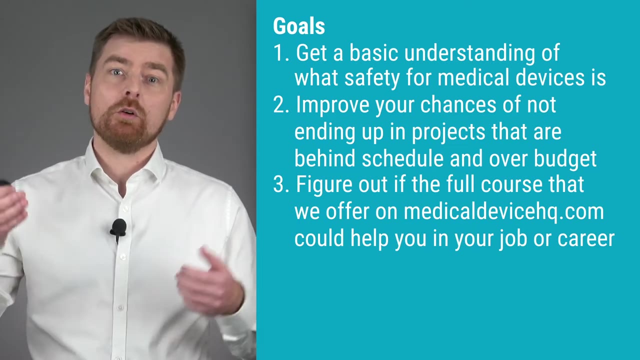 Thank you. The full course is similar to this one, but much more comprehensive, with more in-depth information and quizzes at the end of each topic to test your knowledge and understanding. At the end of the full course, you will also receive a course certificate, which many auditors will be looking for. 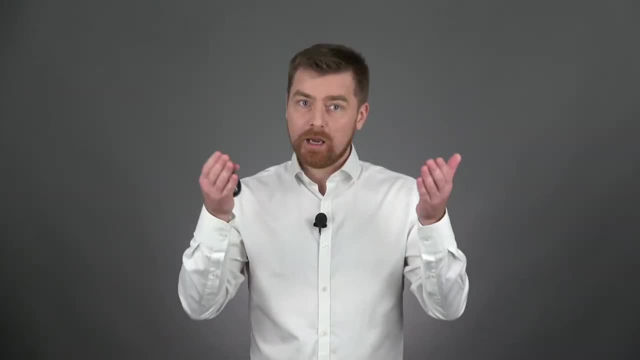 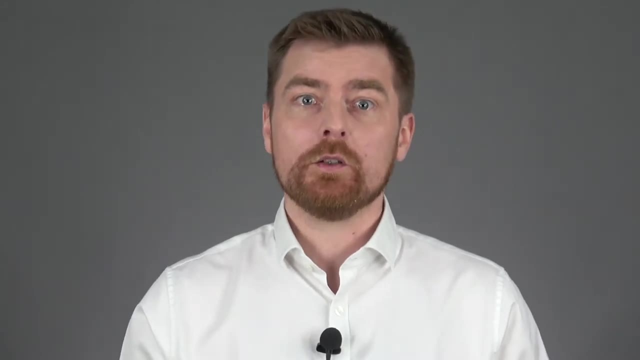 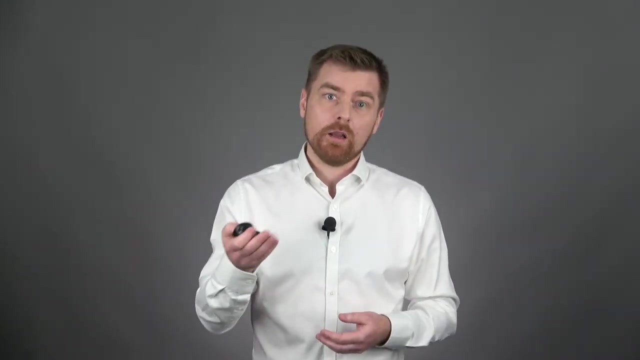 All manufacturers of medical devices aim to ensure that their products are safe and effective. Also, it is a regulatory requirement for every medical device. It is a regulatory requirement for any market where you wish to sell your product. Considering the diversity of medical devices, how they are used and the technologies they employ, this can be challenging. 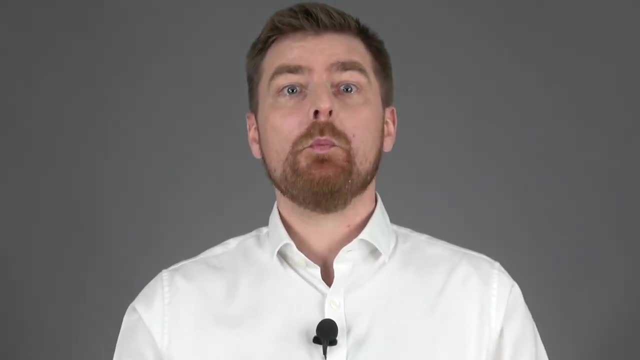 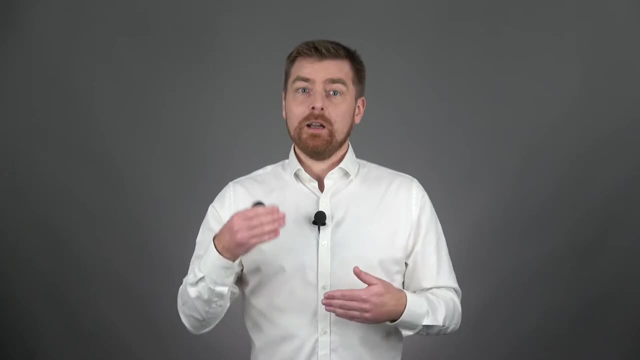 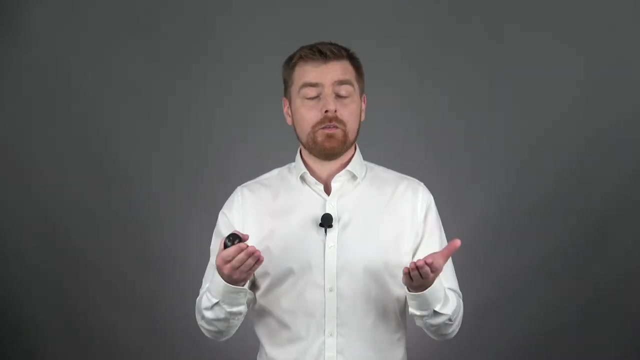 Therefore, standards have been developed to help manufacturers, test houses and regulators. In this part, I will show you how the standards for electrical medical devices are structured. I will try to do this so you can navigate the standards and identify the relevant requirements. 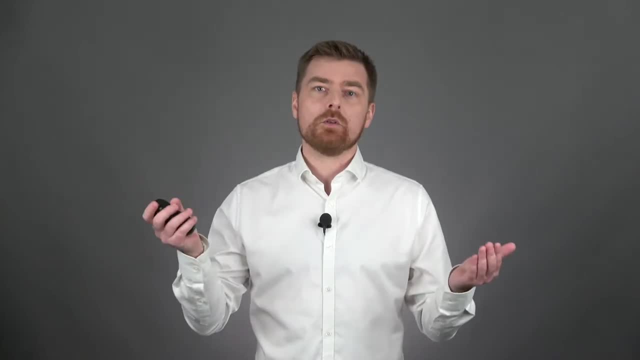 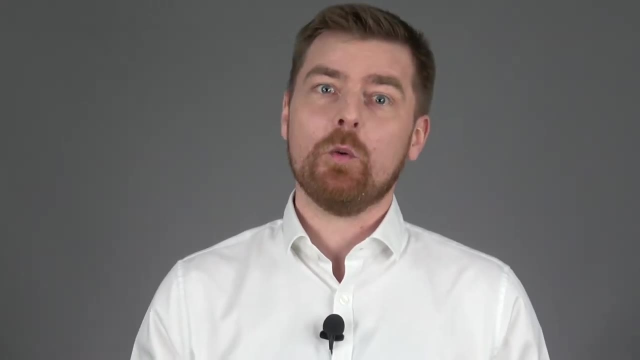 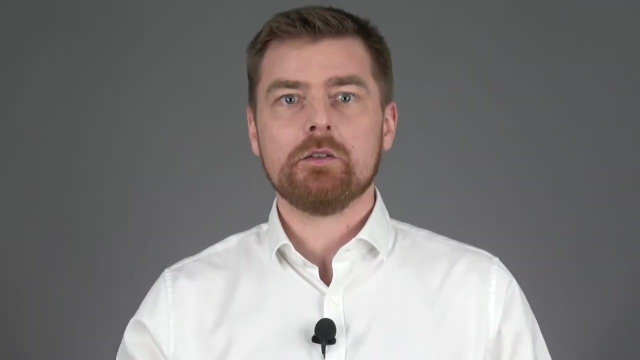 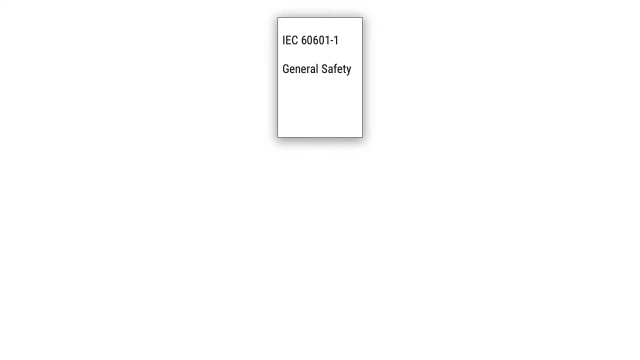 Without having to read many thousands of pages. All these standards in combination define what is called basic safety and essential performance for different types of devices. I will help you navigate these requirements and find the standards relevant to your product. The general standard relevant for safety for electrical medical devices is IEC 60601-1.. 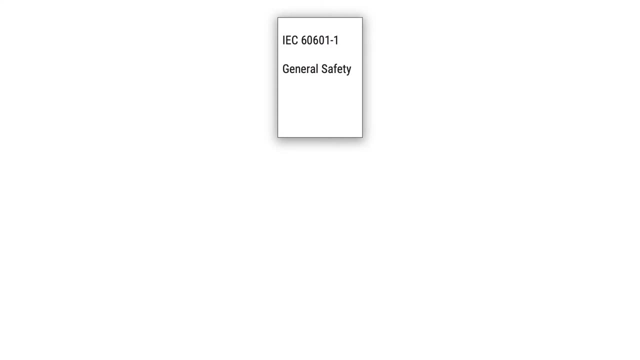 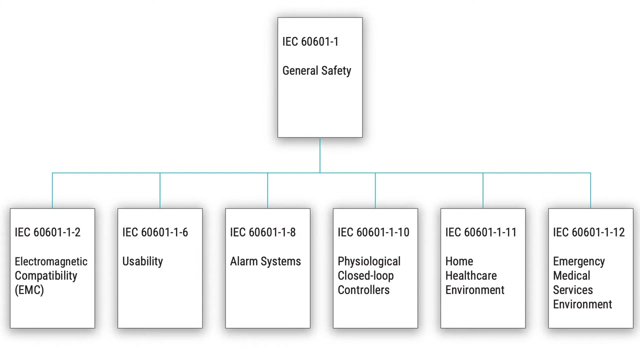 This standard specifies general requirements for basic safety and essential performance. The general standard is an umbrella standard based on collateral standards and particular standards. The collateral standards specify general requirements applicable to subgroups of devices, as well as specific characteristics of devices not covered by the general standard. 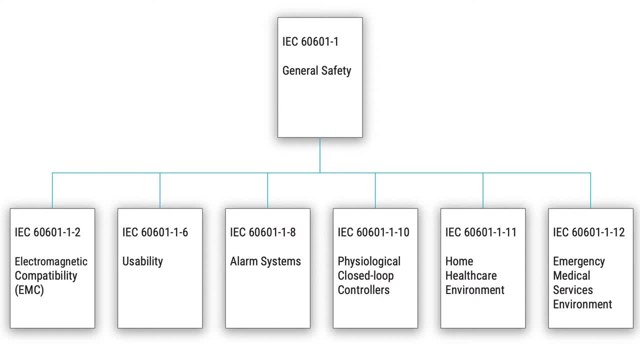 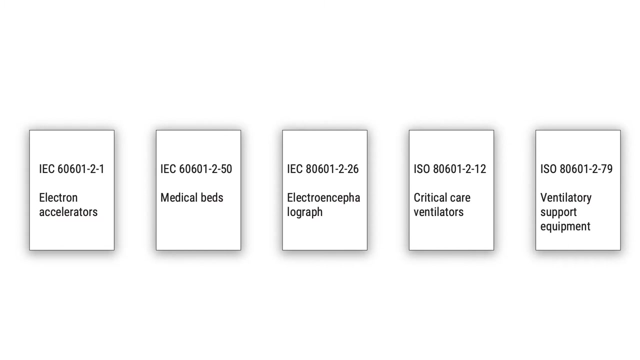 The topics of the collateral standards include electromagnetic compatibility, usability alarms, closed-loop controllers, home healthcare and EMS. In principle, each of these collateral standards apply in parallel with the general standard. In addition to the general standard and the collateral standards, we also have particular standards. 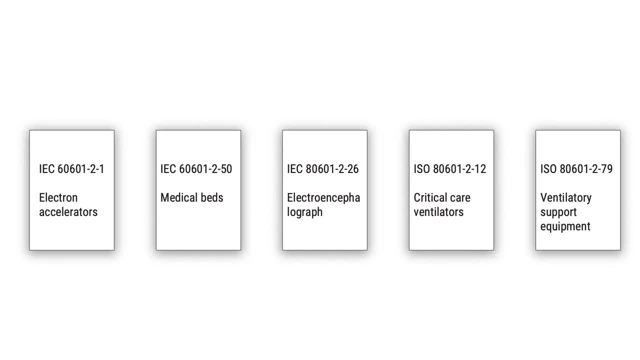 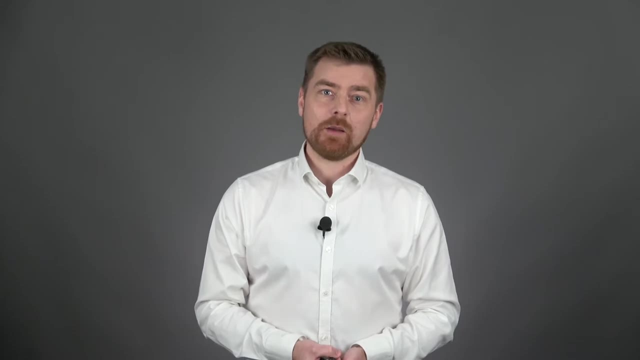 Each of these apply to a very specific type of product. The particular standards may modify, replace or delete requirements contain in the general and the collateral standards. As the standards apply to electrical medical devices having an applied part or a patient connection, you can imagine they define requirements for a lot of hazards. 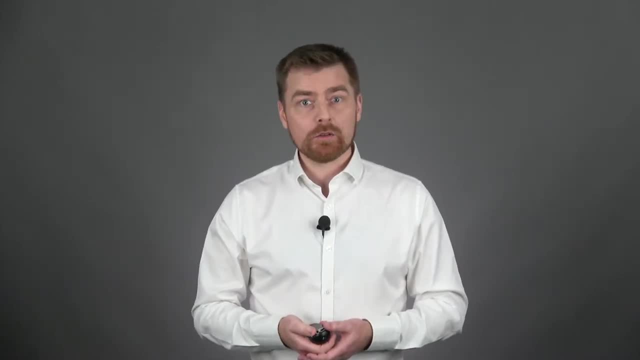 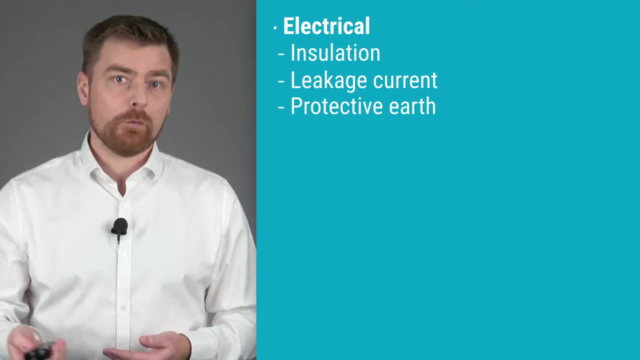 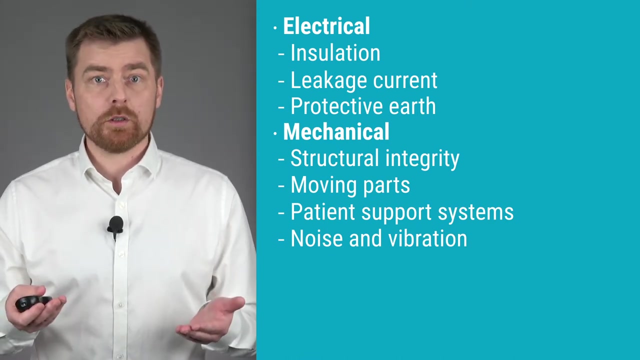 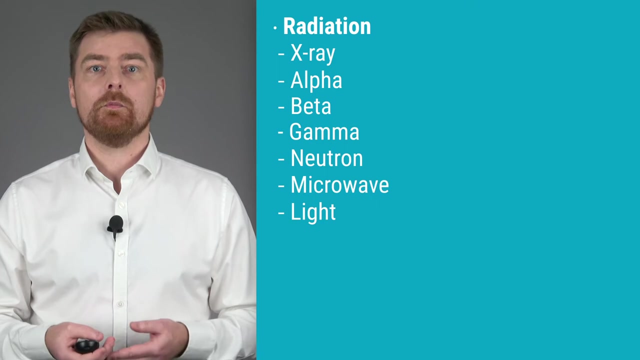 Some requirements are more detailed than others. The requirements include electrical requirements, including insulation, leakage, current protective earth. Mechanical requirements include structural integrity, moving parts, patient support systems, noise and vibration. Radiation requirements include x-ray, alpha, beta, gamma, neutron, microwave and light radiation. 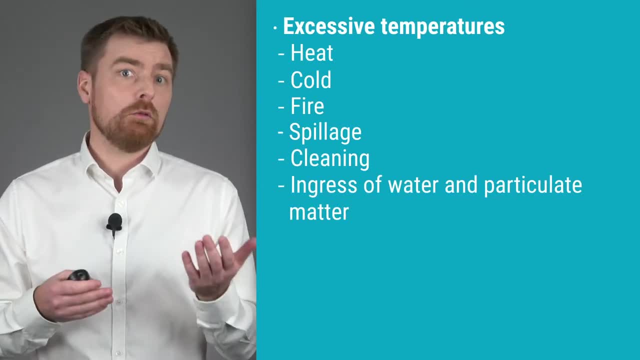 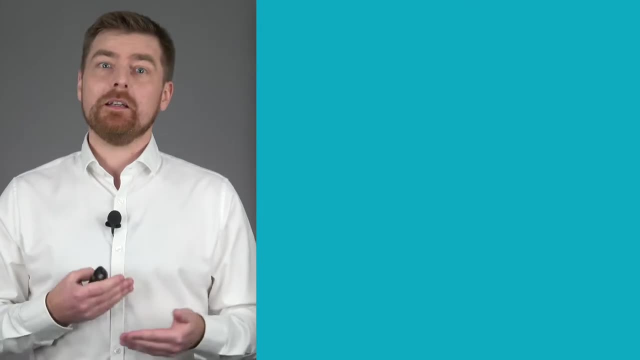 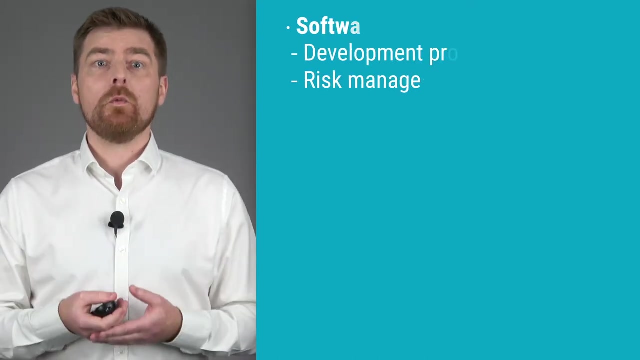 Temperature and other hazards include heat, cold, fire, spillage, cleaning, ingress of water and particulate matter. Use-related requirements include usability, home healthcare alarms and health care Alarms and hazardous outputs, Software requirements for the development process and risk management. 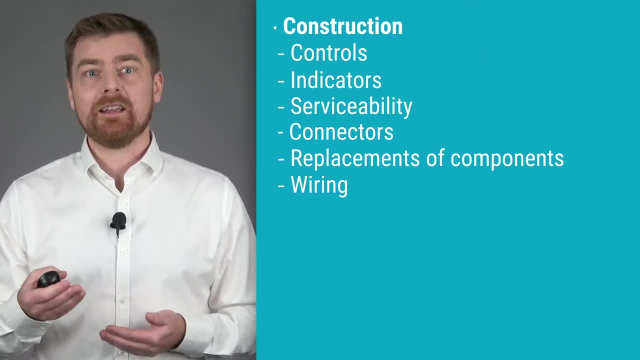 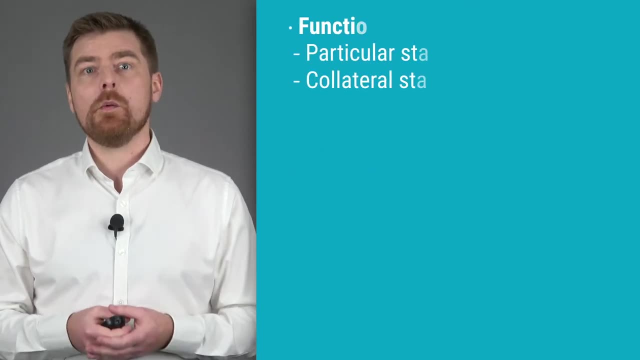 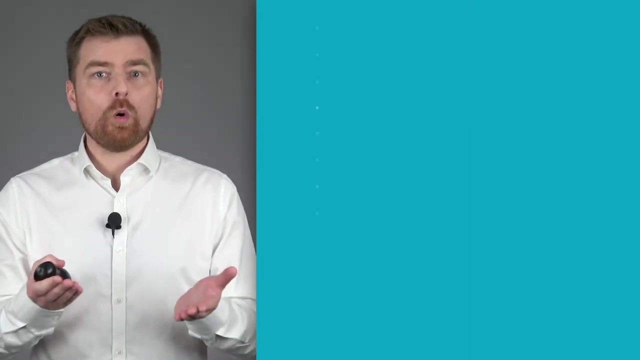 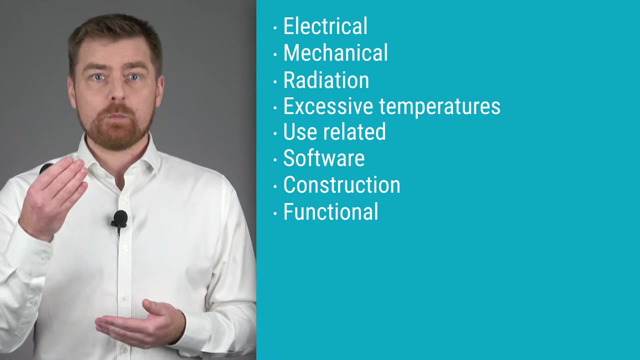 Constructual requirements relate to controls, indicators, serviceability, connectors, replacement of components and wiring. Functional requirements are often defined in particular standards and in some of the collateral standards. All these requirements and other hazards relevant to your device need to be identified and managed through the risk management process. 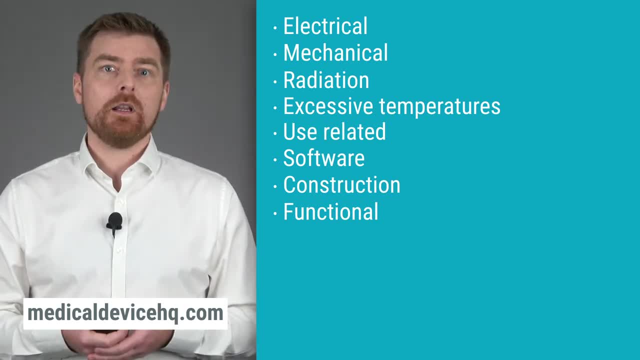 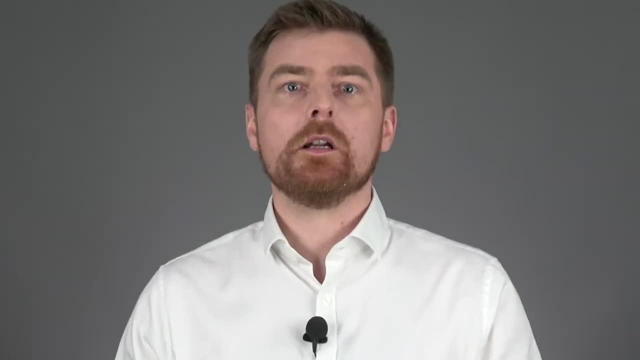 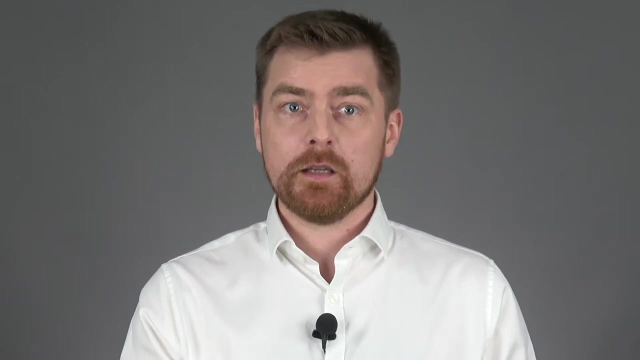 See our course on risk management at medicaldevicehqcom to find out more about risk management in particular. So if your medical device falls within the scope of the 60601-1,, you are going to have to pay attention to all these requirements. 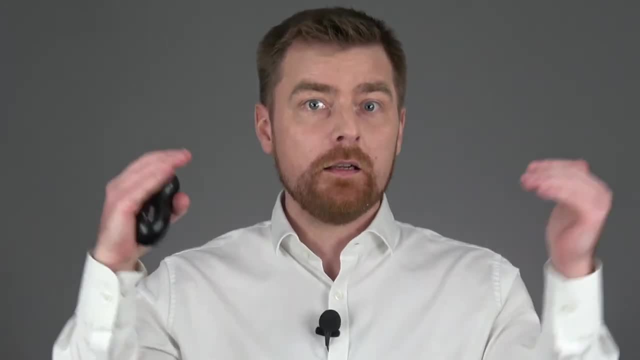 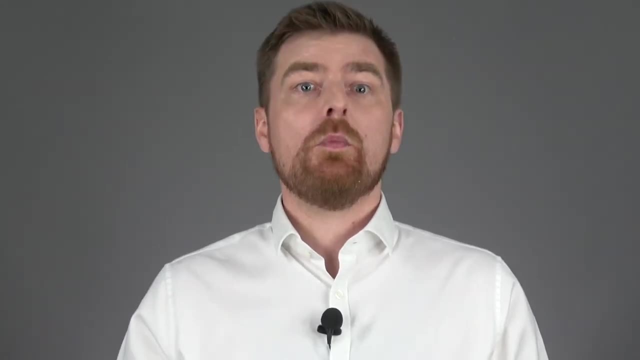 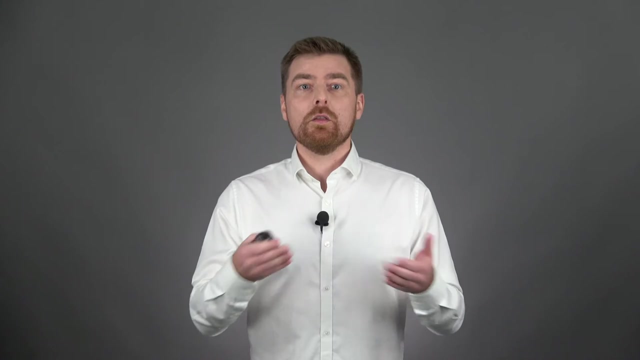 and reach at least the levels defined in this course, Because if you don't, not only do you risk injuring people, but you are also likely to not meet the legal requirements for placing your product on the market. The goal with all of this is to ensure basic safety and essential performance. 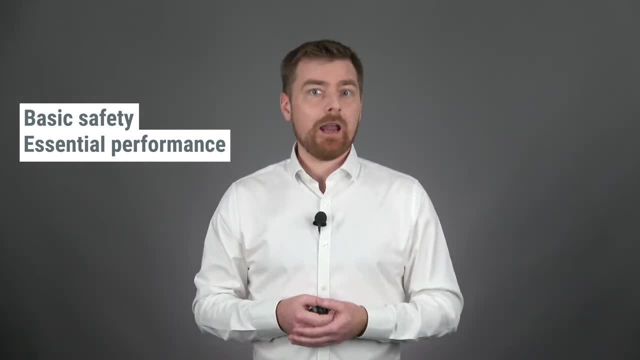 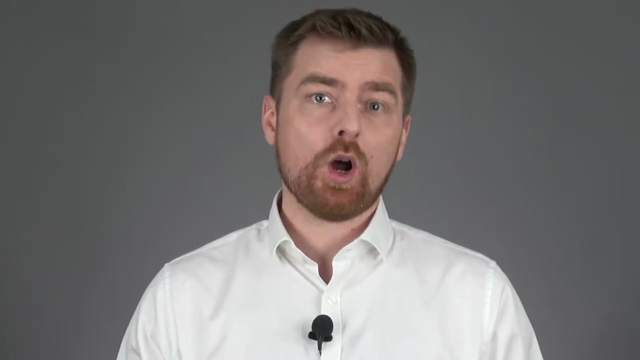 Which basically means that patients and other users shall have freedom from unacceptable risk. Remember, the goal was to get an understanding of risk management, To get an understanding of what basic safety for medical devices is. let's start with the definition of only safety, which comes from ISO 14971.. 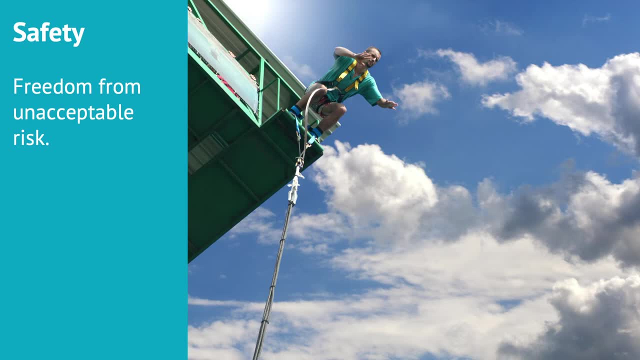 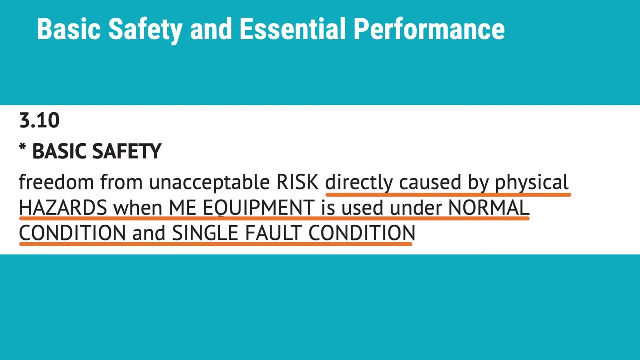 Safety is defined as freedom from unacceptable risk. What is, then, basic safety? Basic safety is to avoid unacceptable risk directly caused by physical hazards when medical electrical equipment is used under normal condition and single fault condition. As you can tell, this is a slightly more narrow concept compared to safety in general. 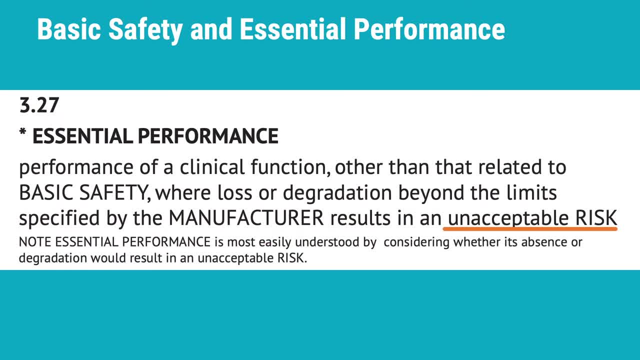 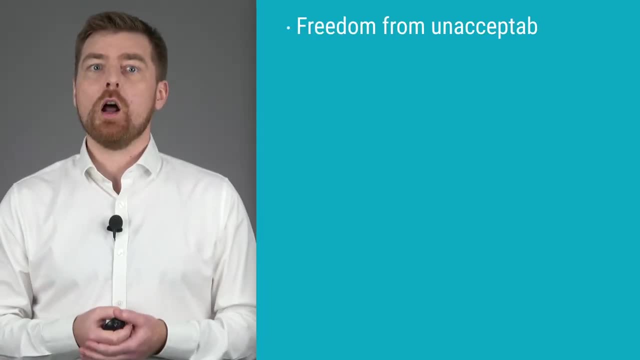 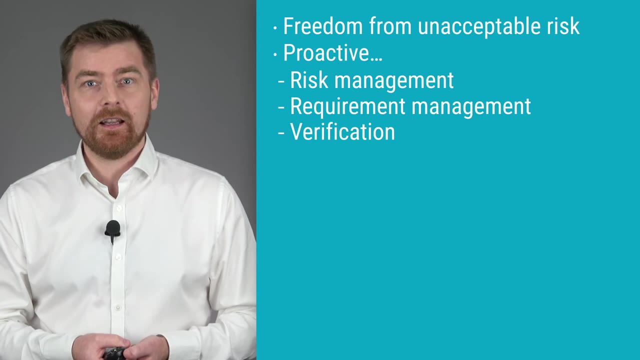 And this is the definition of essential performance, which has the same objective: to avoid unacceptable risk. Now, if you only have one takeaway from this course, let it be this: Freedom from unacceptable risk is achieved through proactive risk management, requirement management and verification during all development phases and thereafter. 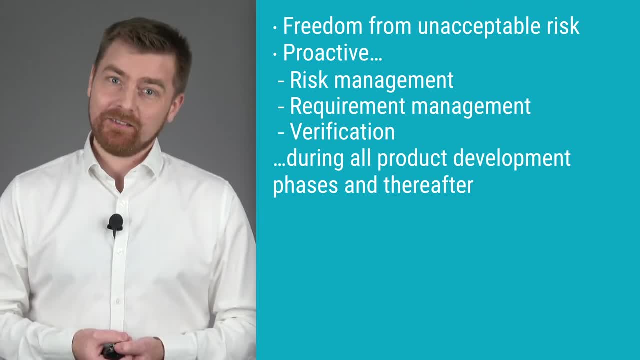 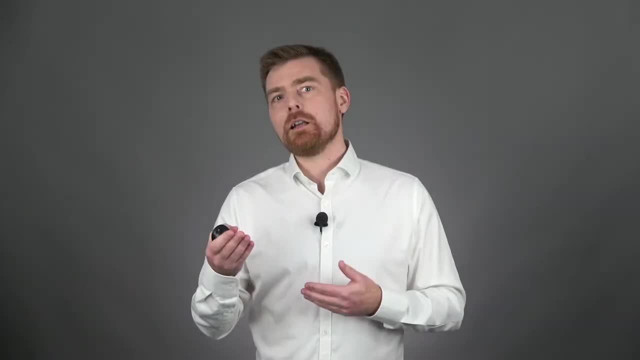 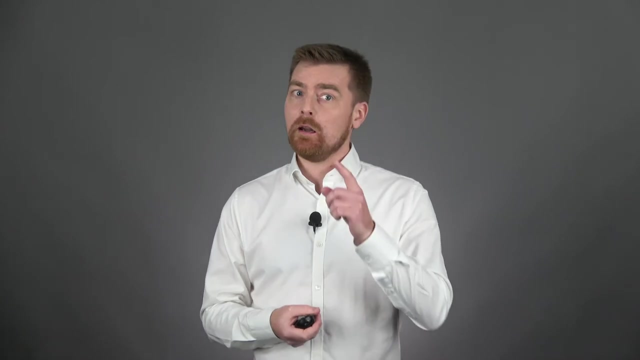 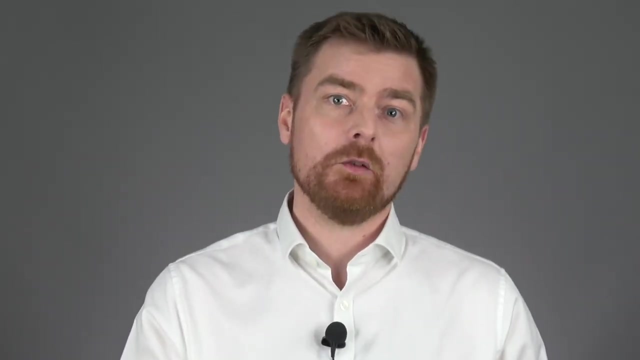 To establish that the device is safe. you should manage all risks relevant for electrical medical devices. Let's now talk about where most manufacturers fail to address safety by design and how you can proactively avoid making the same mistake. This will help you develop safe medical devices in an effective and efficient way. 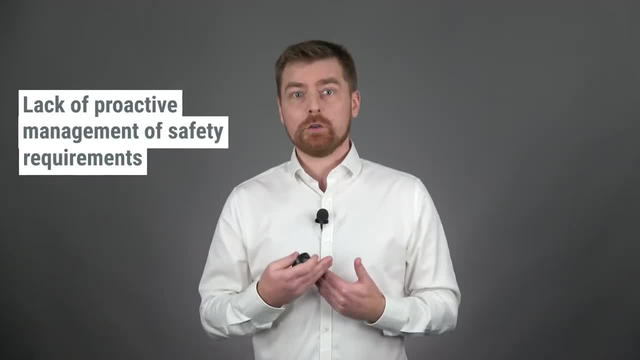 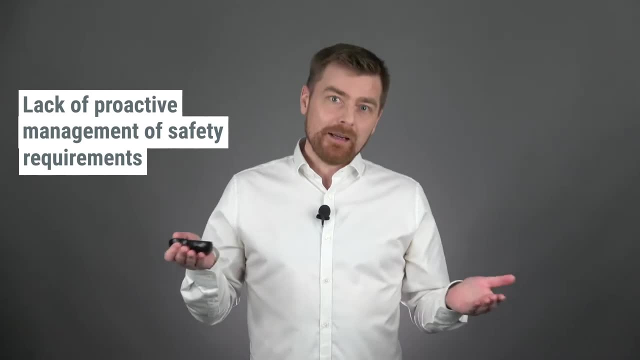 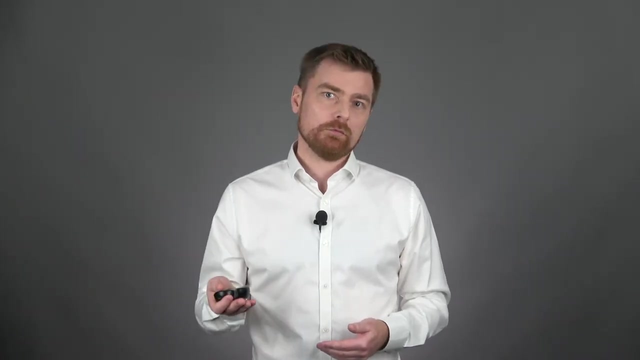 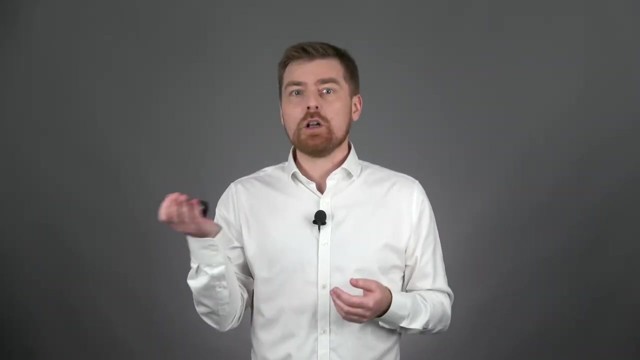 In my experience, the most common problem manufacturers face is the lack of proactive management of these many requirements. Many manufacturers won't spend any significant time on the requirements from 60601-1 until they have sent the medical device to third-party testing and discover that they did not meet one or several requirements. 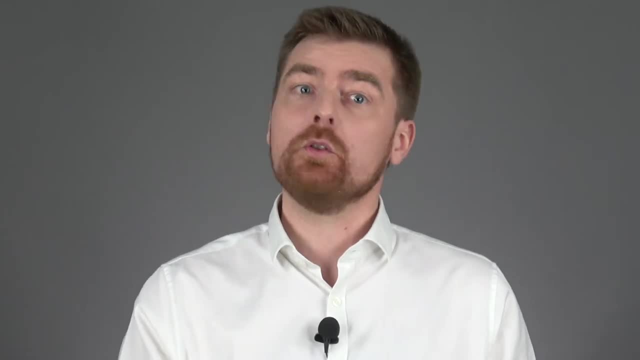 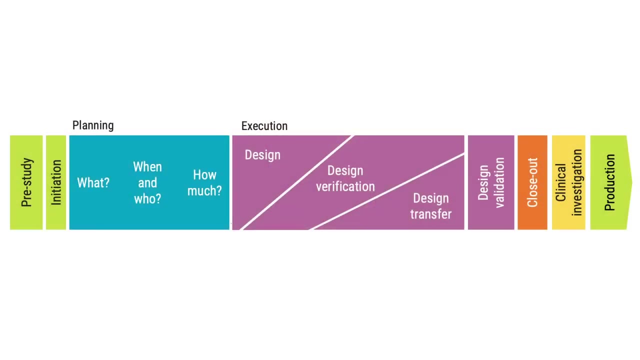 And some of these things you can do yourself to save time and money. This will be discussed further in the full course. Typically, safety-related activities are performed late in the design verification phase or even as late as the design validation phase. This results in failed tests, redesign and retesting, which add costs and delays. 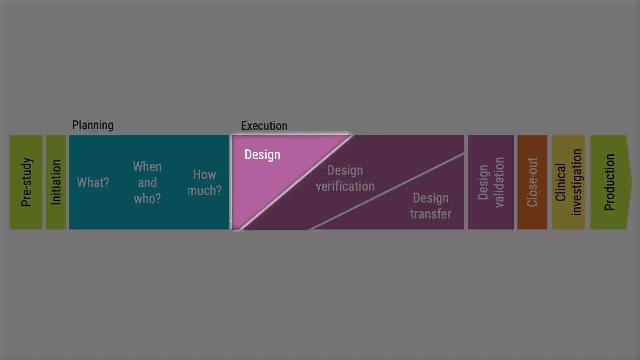 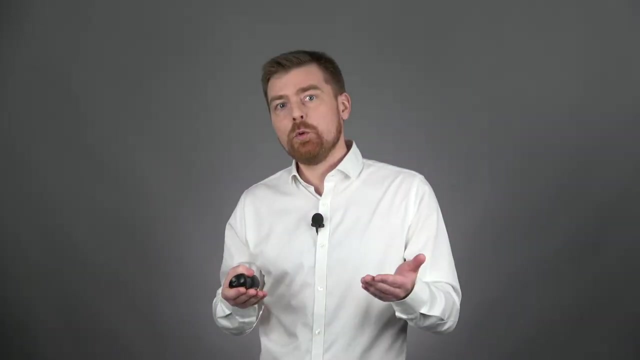 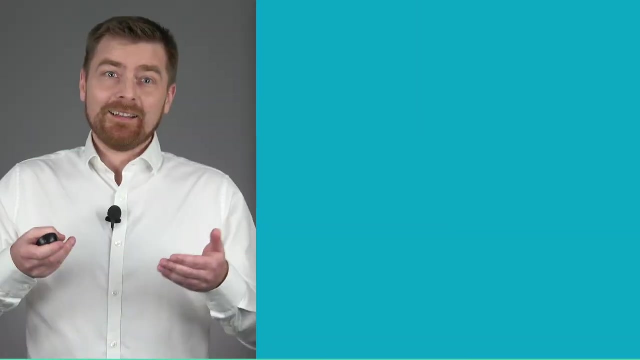 To avoid costly delays, I recommend that you identify the few relevant requirements early during the design phase and decide how the design is going to meet these requirements. As I referred to in the beginning, the key to proactive safety by design is to start early and based on the intended purpose and technologies. 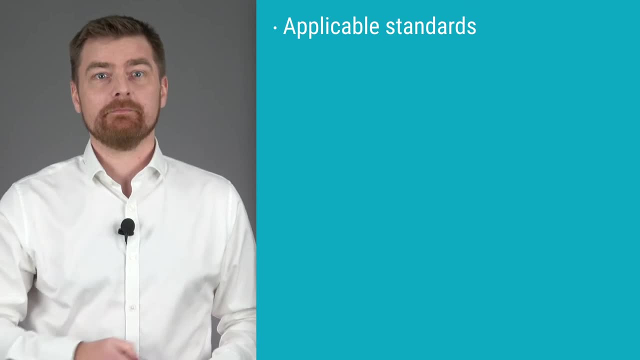 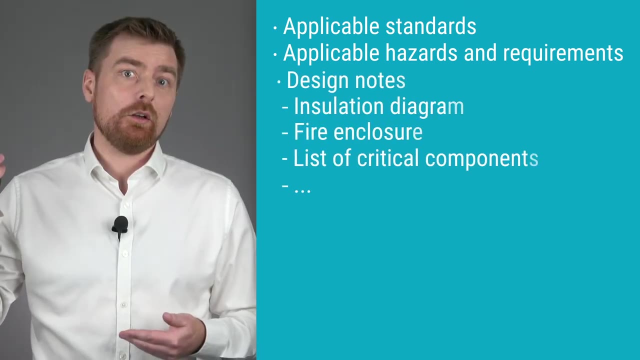 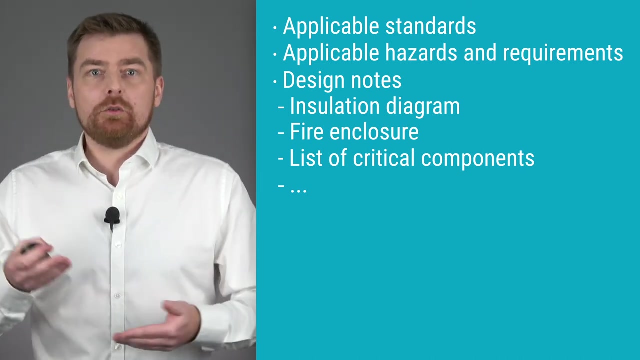 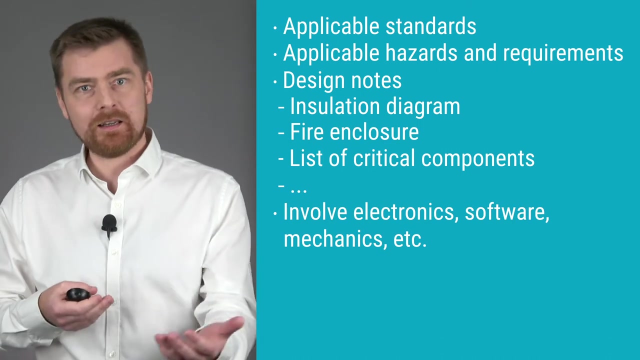 identify which standards are applicable to your device and identify which of the hazards and requirements are applicable to your device, Then document in design notes how the product is designed to be safe. It is critical to do this as a cross-functional team exercise because it is the combination of electronic, mechanic and software solutions. 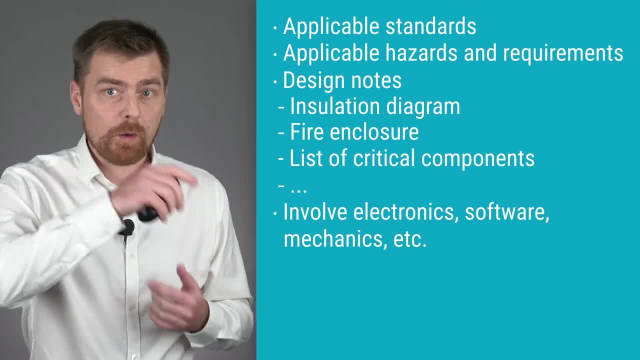 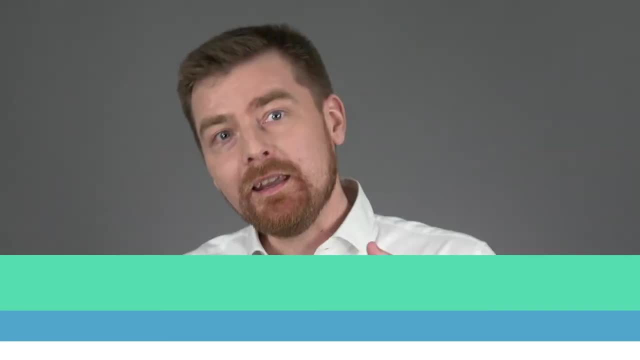 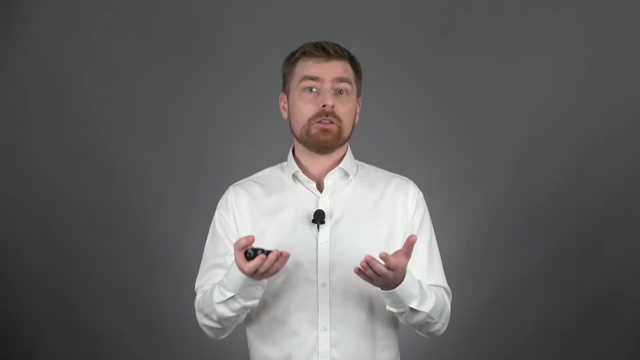 that must meet the requirements. Remember, risk management should be a team effort and safety is a system property. In the beginning I promised you I would share my trick to make safety engineering fun. To be honest, it is very simple. I always try to be curious and start by asking questions. 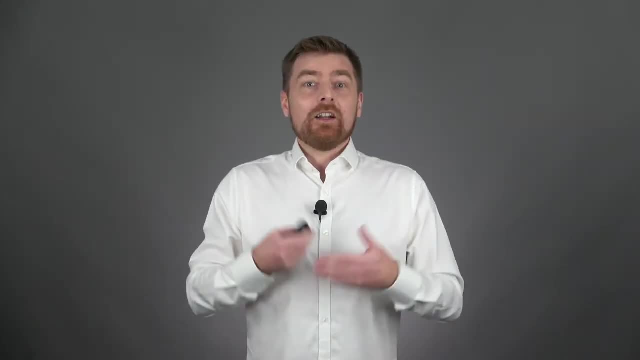 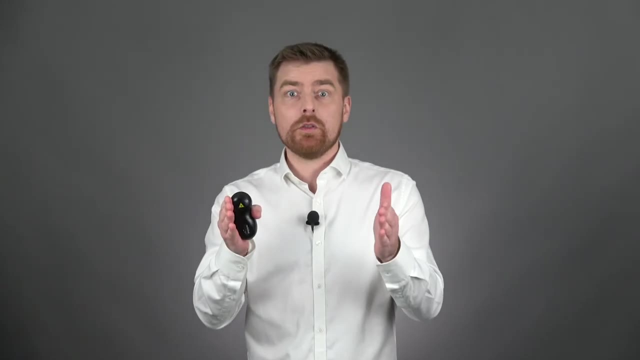 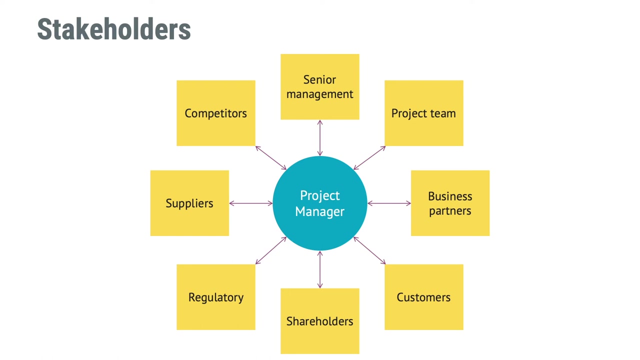 rather than finding solutions. I do this to identify the few features which are critical to the product, And then I focus on these. Next, I ask all stakeholders for their input. This includes team members, management, suppliers and so on. I also consult standards and guidelines to ensure I understand all aspects of the requirements.